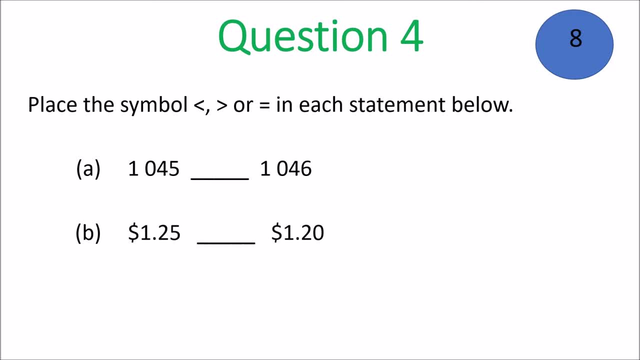 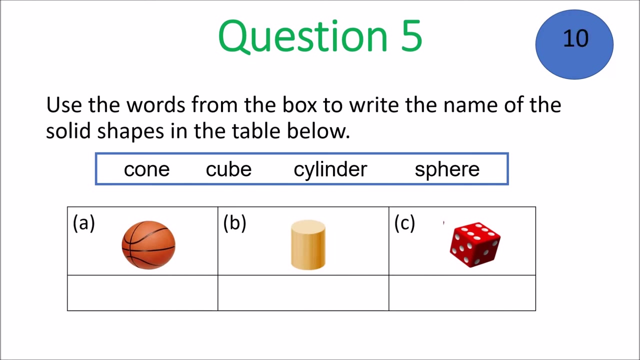 A and then B, A and then B, A and then B, And we move on to question. 5. Use the words from the box to write the name of the solid shapes in the table below: Cone, cube, cylinder square. 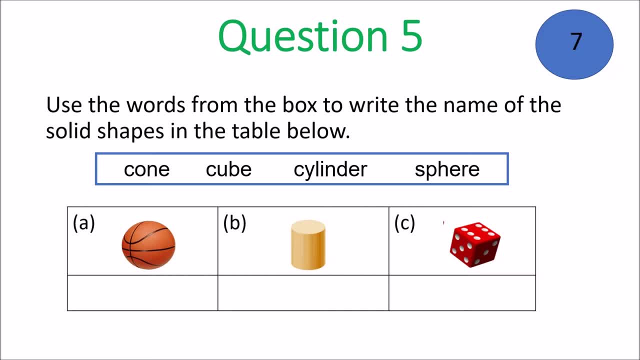 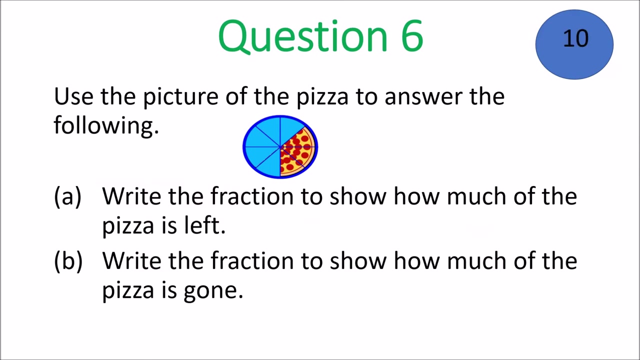 A, B and C And we move on to question 6.. Use the pitch of the piece to write the name of the solid shapes in the table below: B, B and C. A and B, A and B, A and B. 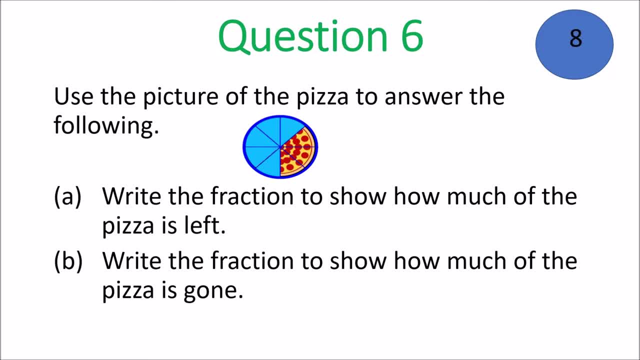 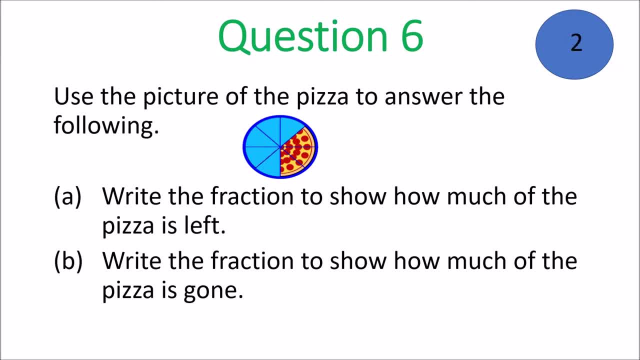 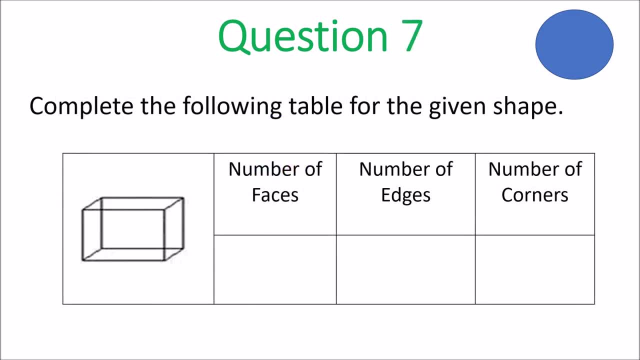 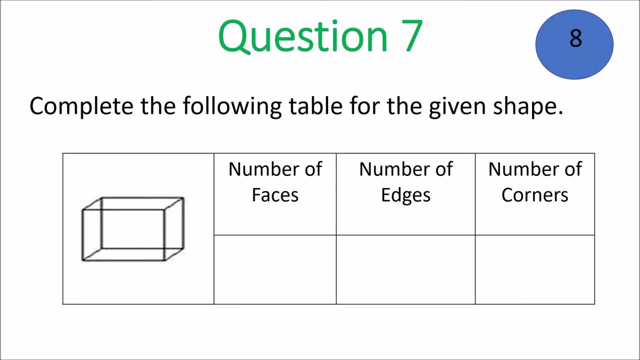 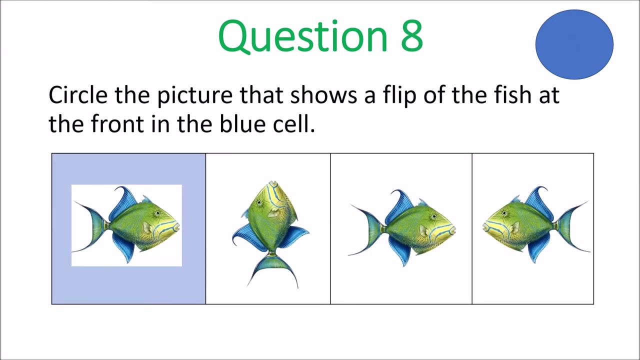 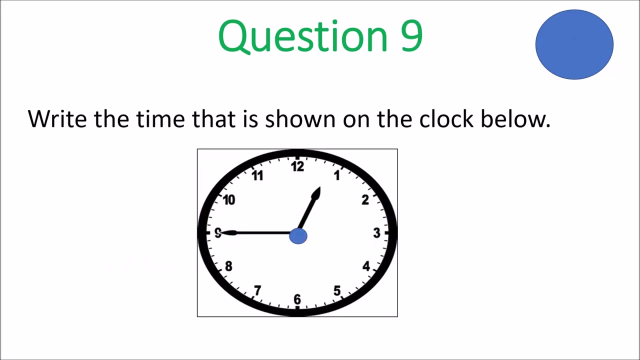 Number of edges and number of corners. Here we go. Question number eight: Recall the picture that shows a flip of the fish at the front in the blue cell. Question nine: Write the time that is shown on the clock below And the final question. 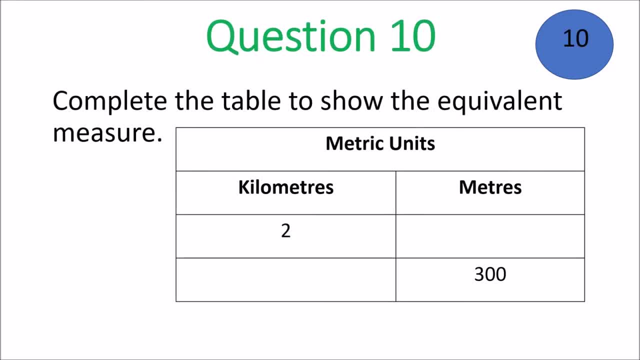 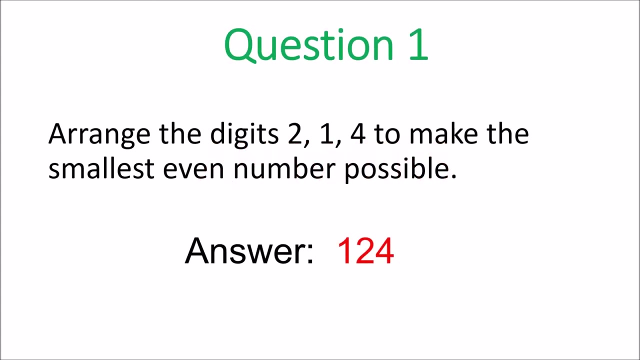 Question ten: Complete the table to show the equivalent measure Your metric units in kilometers and meters. Now we move on Two answers. Please mark and see how many you get correct. Question one: Arrange the digits two, one and four to make the smallest even number possible. 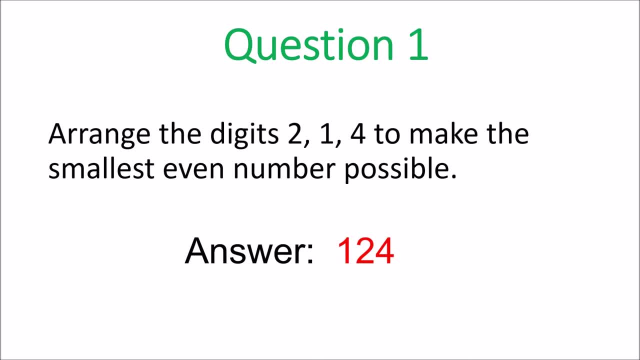 Add numbers: One hundred twenty-four, One hundred twenty-four. Okay, you have to put the two and then the four. If it can't be one forty-two, that would be bigger. So the smallest is one, two, four. The one has to be at the front. 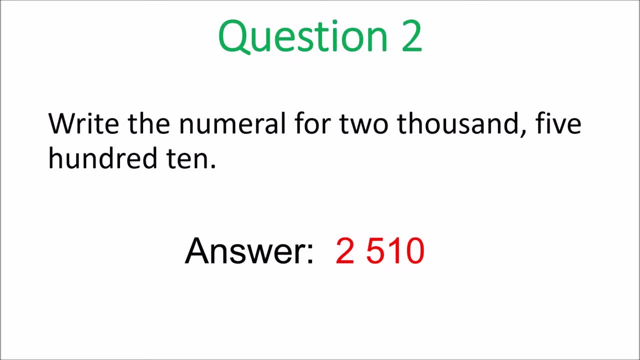 Hope you got that correct. Number two: Write the number for two thousand five hundred ten. Two five, one, zero. That's it right there. Two thousand five hundred ten. Okay, So you have to put a zero in the ones place. 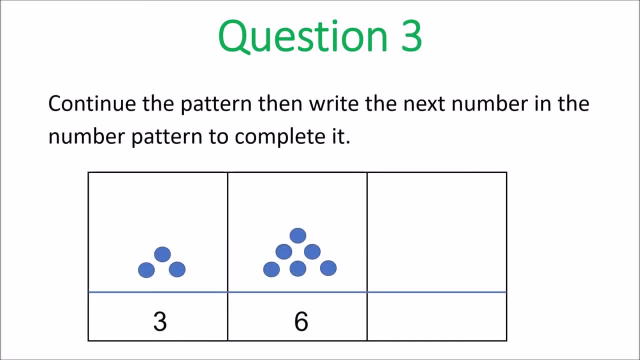 Once you got that, you're okay. Question three: Continue the pattern and write the next number in the number pattern to complete it. Yeah, so it's one on the top and the bottom of that. you put two under that, you're going. 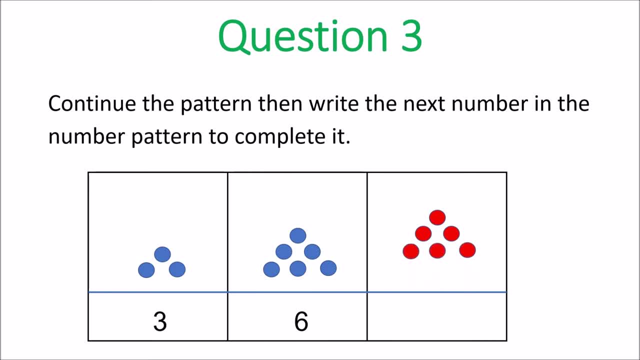 to put three under that. how many do you put Four? Add them up, Count them up. How many do you get Four? three, two and one. Yeah, Four, Yes, you get ten. So it's three, six and ten. 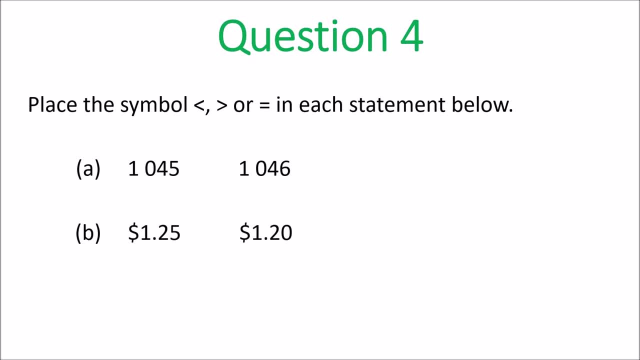 Question four: Place the symbol less than greater than equal to, So A one thousand forty-five and one thousand forty-six. Which one is smaller? One thousand forty-five, So you'll point it to: one thousand forty-five, Dollar twenty-five and a dollar twenty. 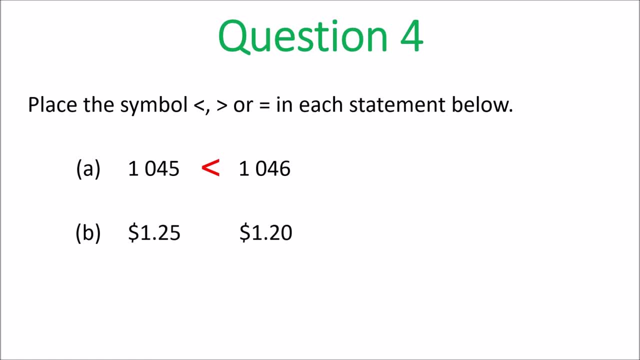 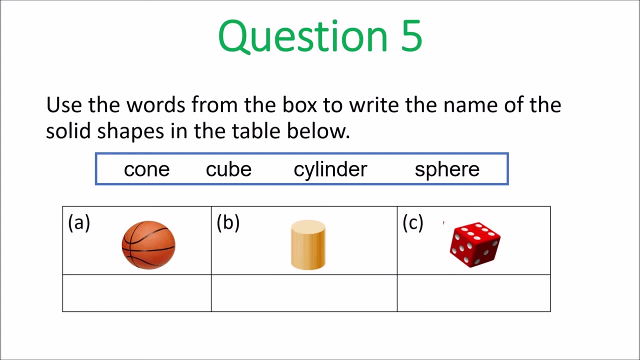 Which one is smaller? Yes, dollar twenty. So you'll point it to a dollar twenty. So we'll read: a dollar twenty-five is greater than a dollar twenty. for B, Question five: Use the words from the box to write the name of the solid shapes in the table below. 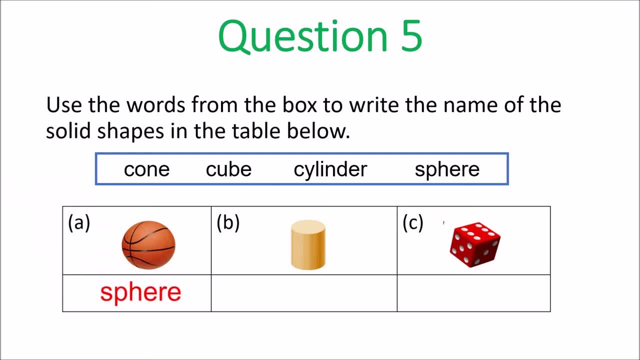 And you had cone, cube, cylinder square. So that's a square, The ball is a square. Next one: What's B? Right? It's a cylinder Can shape Cylinder. Final one: See if you got this. 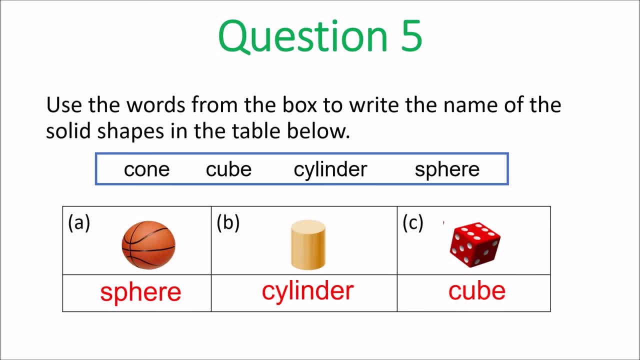 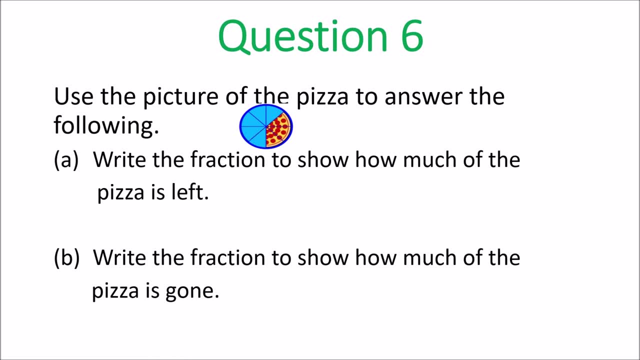 Cube: Yes, It's a cube. Hope you got this. Hope you got all of those correct guys. Question six: Use the picture of the pizza to answer the following: Write a fraction to show how much of the pizza is left. 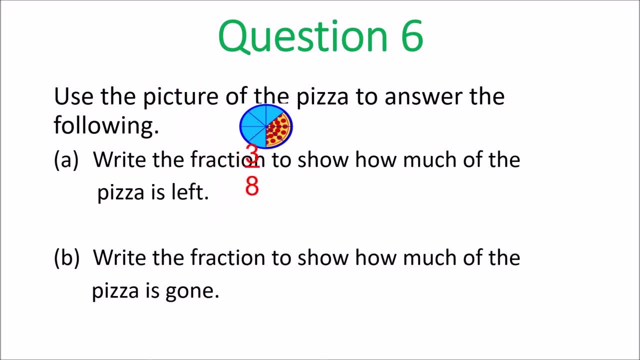 So how much of that pizza do you see there? Three eighths, That's correct. Three pieces left and there were eight pieces altogether. What fraction to show how much is gone? Five eighths, Yes, because five pieces are gone and there were eight pieces altogether. 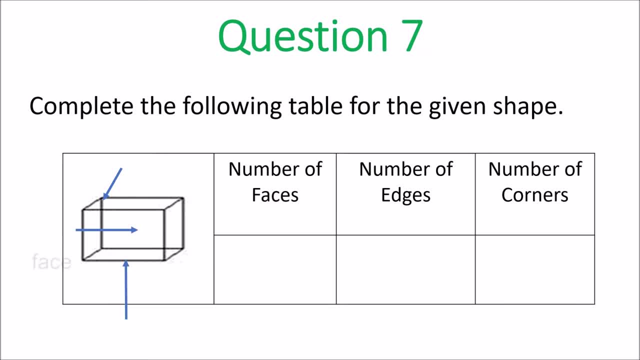 Question seven: Complete the following table: for the given shape, Number of faces: A face would be a flat surface. How many flat surfaces? Six Edge would be the lines. How many of those lines? Count them up. Twelve of those lines. 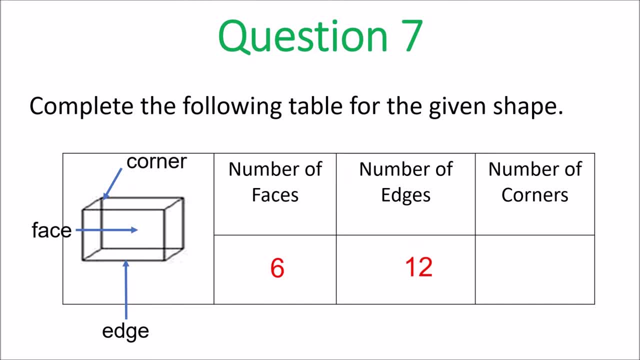 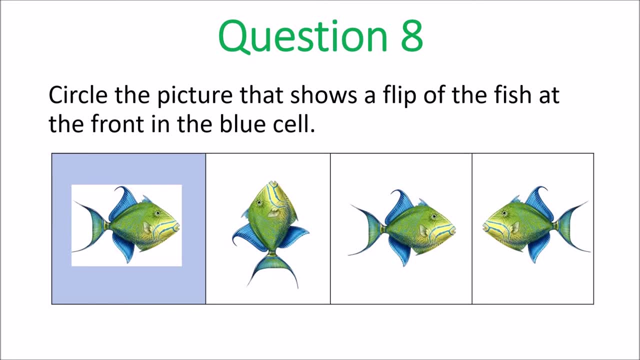 And the corner or the vertices would be where two edges meet. And how many do you have? Four on the top, four on the bottom, Eight. And a circle is a picture that shows a flip of the fish at the front in the blue. 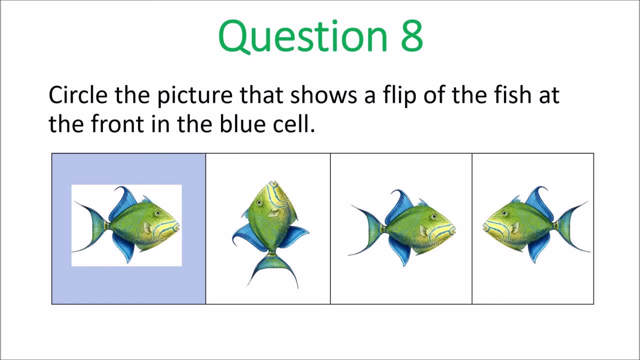 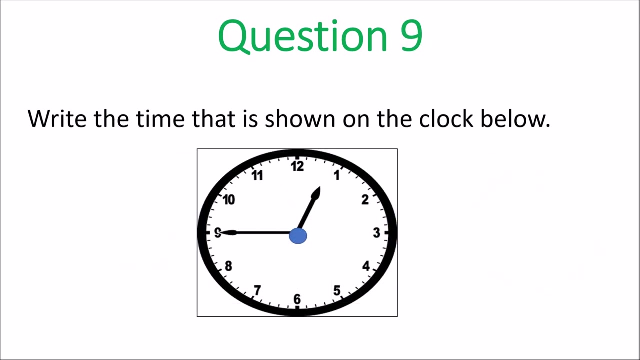 cell. Which one is it? Remember, you want a flip and it would be that last one. That last one is a flip of the fish at the front, Turns at the opposite direction And question nine. Write the time that is shown on the clock below: 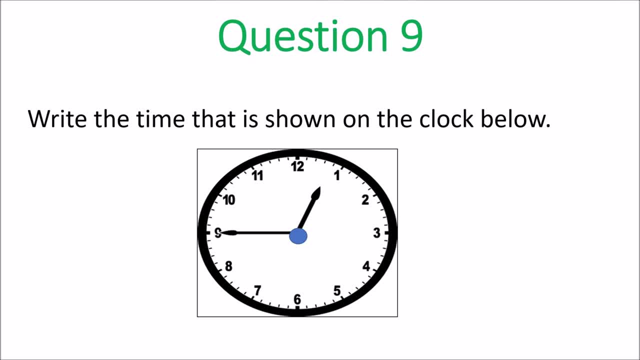 So it's nine. two ways to do it: 1245. or you could have said 15 minutes to 1, 15 minutes before one. it's another way. you could have said that any one of those in your correct question, 10, last one, complete the table, show the equivalent measure. so it's two.